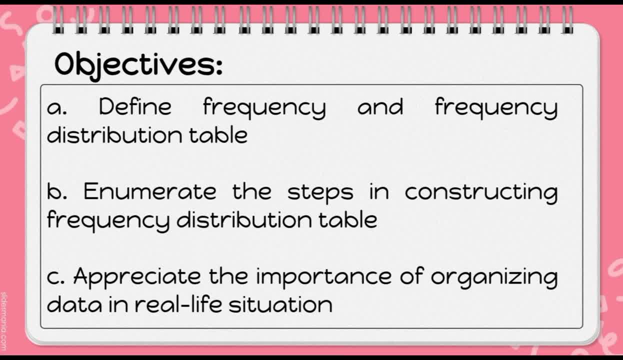 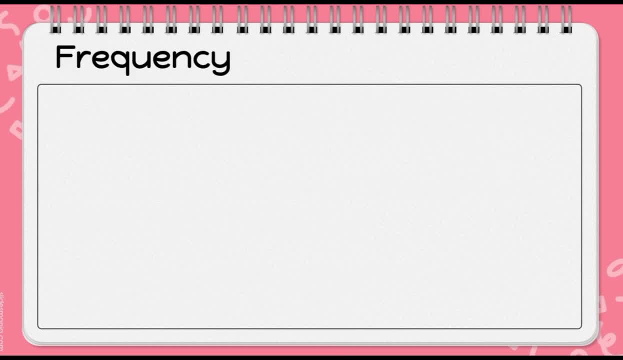 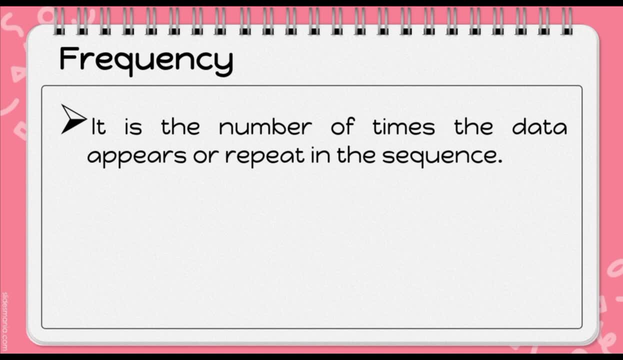 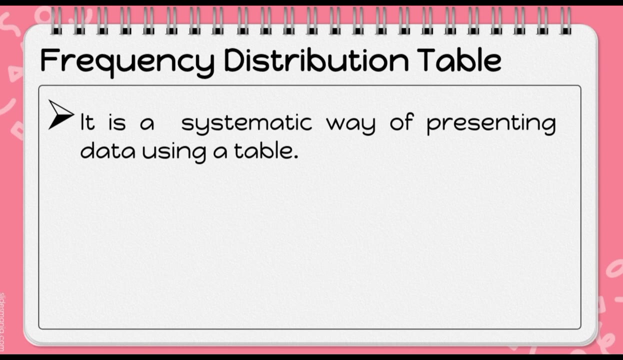 frequency distribution table and, lastly, we have appreciate the importance of organizing data in real-life situation. so what is frequency? so when you say frequency, it is the number of times the data appears or repeat in the sequence, and when we say frequency distribution table, so it is a systematic way of 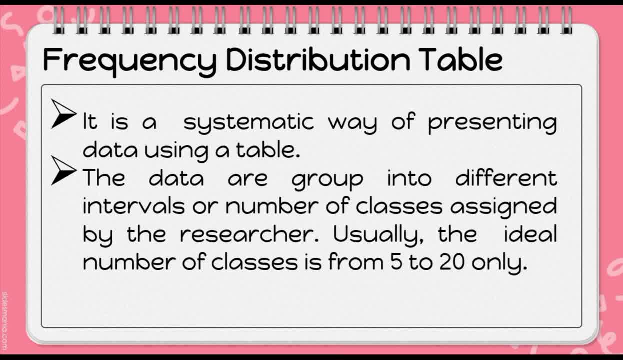 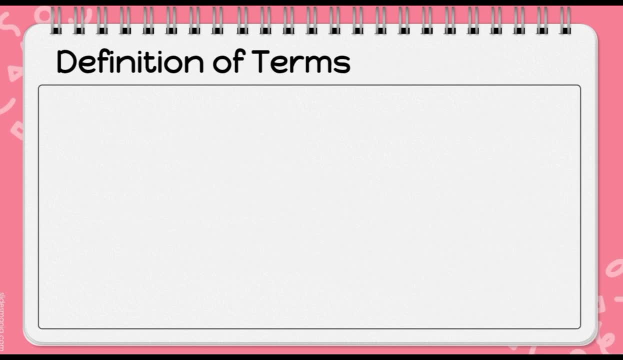 presenting data using a table. so the data are grouped into different intervals or number of classes assigned by the researcher. so usually the ideal number of classes is from 5 to 20 only. so we have important terms that we need to know, especially in constructing frequency distribution table. so first, 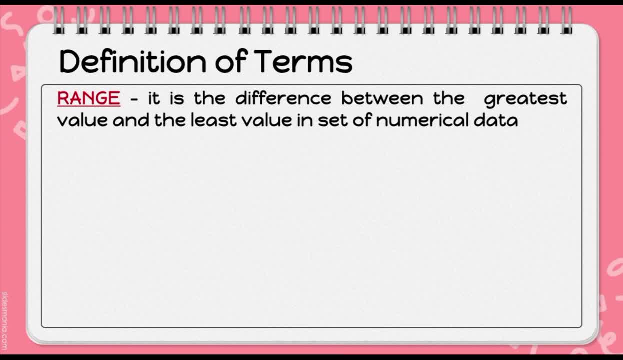 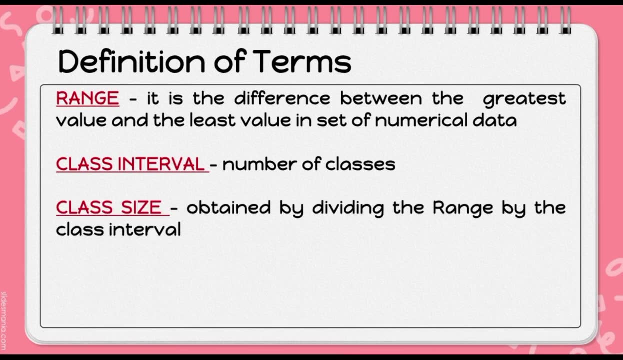 is: we have range. so when we say range, it is the difference between the greatest value and the least value in set of numerical data. second, we have class interval. so when we say class interval, it is the number of classes. and next we have class size. so we say class size, it is obtained by dividing the range by the. 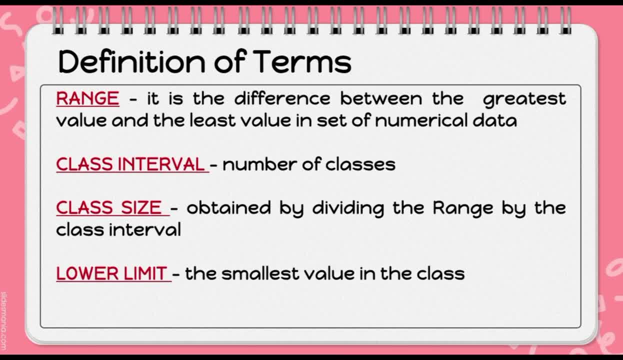 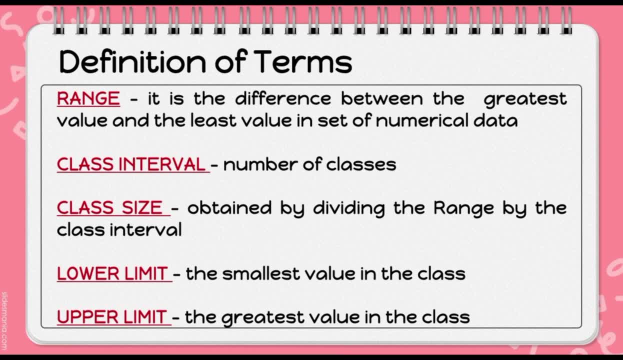 class interval. third is lower limit. so it is the smallest value in the class and the upper limit we have the greatest value in the class. so you have to familiarize these terms because we will be using that one as we go along to our discussion. moving on to steps in constructing, 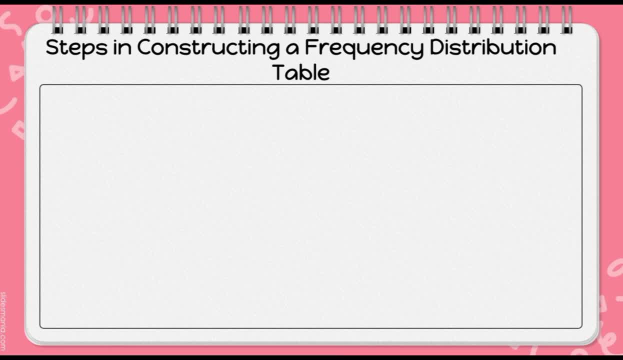 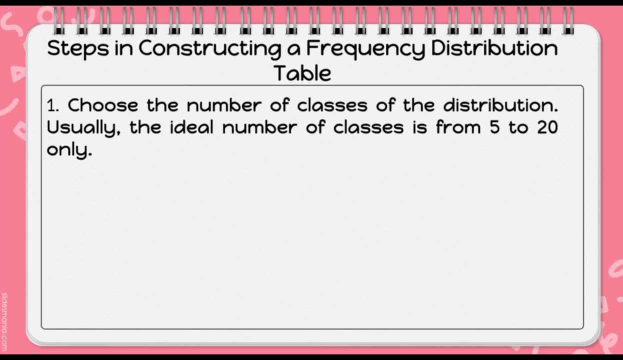 a frequency distribution table. so we will be using this example. so here are the savings Kim has in the month of May. so first step: we have choose the number of classes of the distribution. so usually the ideal number of classes is from 5 to 20 only, as what I have said earlier. so in our 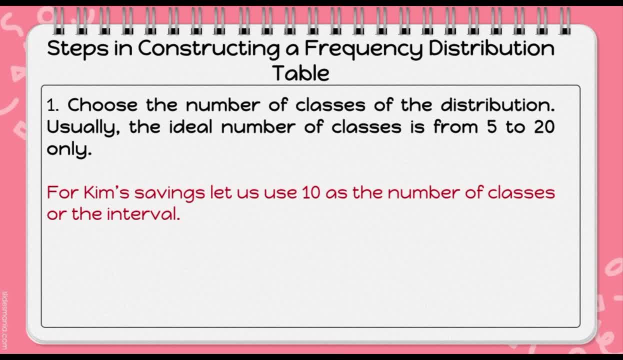 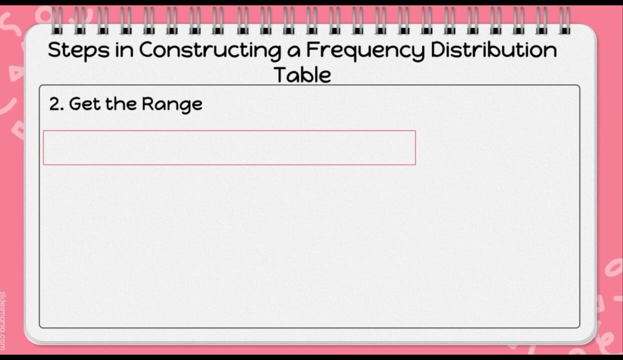 example. so for Kim savings. so let us use 10 as the number of classes or the interval, so in this example. so I will be the one to give you the class interval, so that we will have the same answer later on. so therefore, our class interval: 10. for our second step, we have get the range. again, when we say range, it is the. 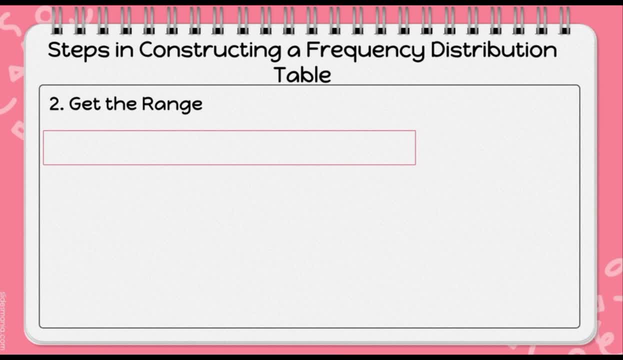 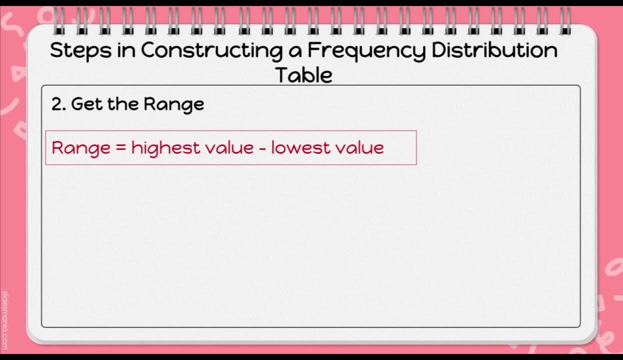 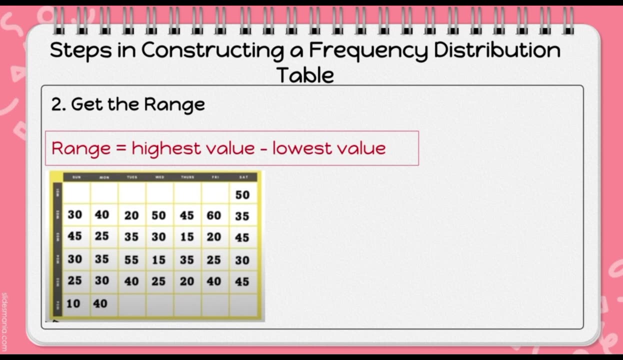 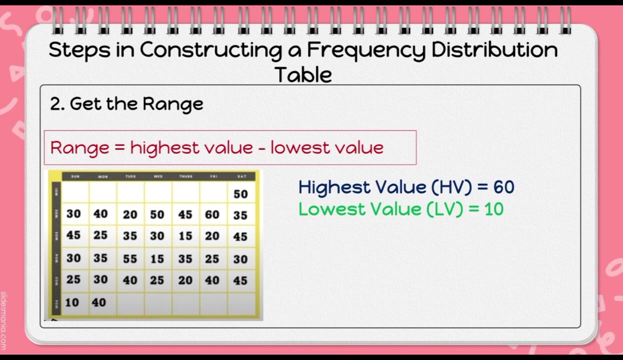 difference between the highest value and the lowest value. so we have this formula: range is equal to the highest value minus the lowest value. so here in our example, so our highest value is equal to 60 and our lowest value is equal to 10. so in applying the formula, in getting the range, we have highest value minus. 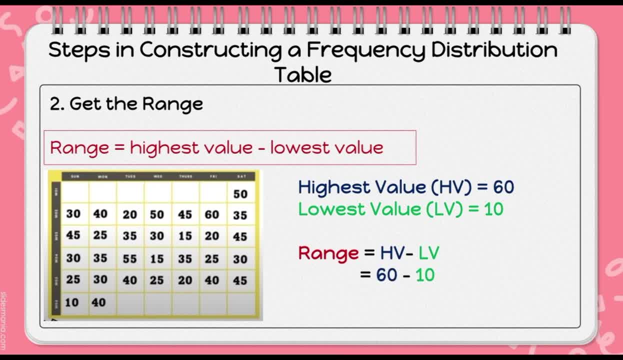 the lowest value. so again, our highest value is equal to 60 minus our lowest value is equal to 10. so 60 minus 10 is equal to 50. therefore the volume of our range numberле will be $600. if you multiply that value by 10, you can see that is. 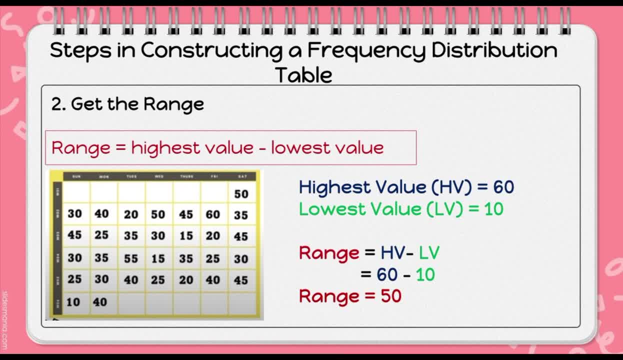 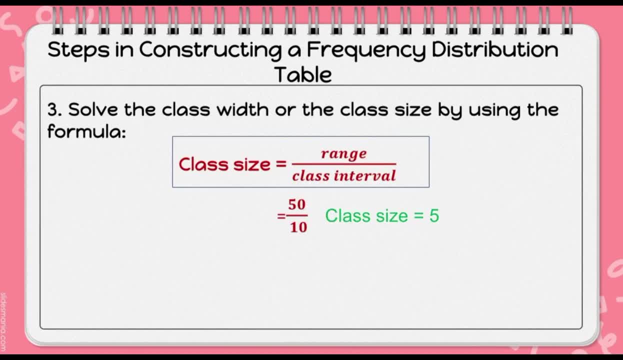 going to be almost와 60 minus. our highest value is equal. 60 is equal to, 60 is equal to value of our range is equal to 50. so remember this one because we will be using this in our next step. alright for our third step. we have solve the class. 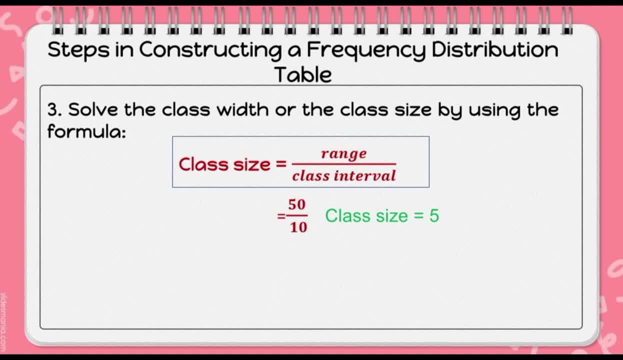 width or the class size by using the formula. so we have this formula in solving for class size. so class size is equal to the range divided by the class interval, since we have already solved for the range. so we simply substitute the value of our range, which is 50 right, divided by our class interval, which is 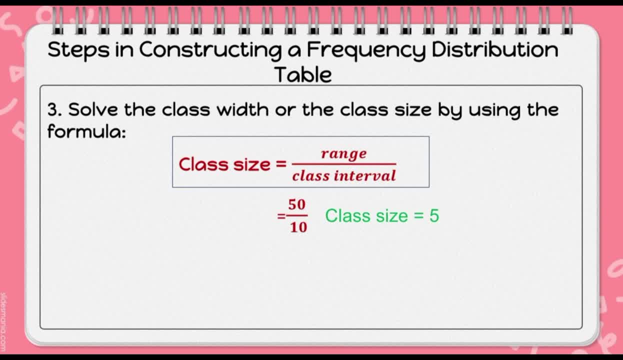 10, as what I have said earlier, that we will be using 10 as our class interval. so 50 divided by 10 is equal to 5. so therefore, our class size is equal to 5. by the way, if you want to know how to solve for class size, you need to know. 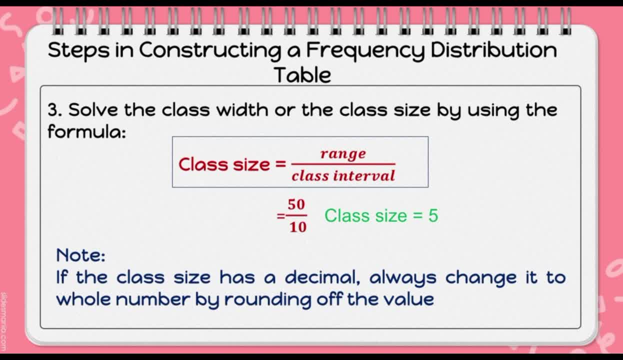 by the way, if you want to know how to solve for class size, you need to know. by the way, you have to take note this one: if the class size has a decimal, always change it to whole number by rounding off the value. so you have to remember the rules in rounding off a number, for example, 0.4 and below. so our 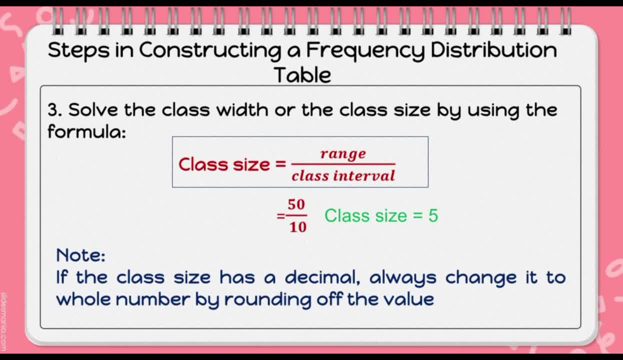 whole number is still the same. for example, 4.4 is equal to 4 and 0.5 and above we will add 1 to our whole number, for example, 4.5, so 4.5 will become 5, because we will add 1 to our whole number, which is 4. so 4 plus 1 is equal to 5. I know. 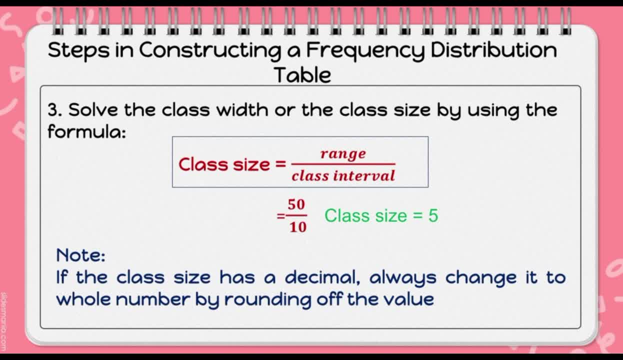 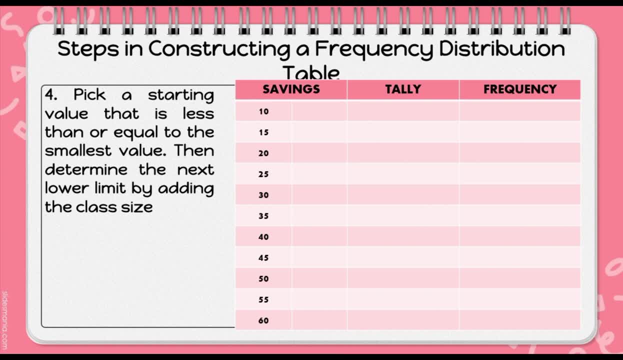 you know this one because this is already tackled in your previous lesson. in rounding off, a number, all right, for our fourth step, we have to pick a starting value that is less than or equal to the smallest value, then determine the next lower limit by adding the class size. so here in our example, 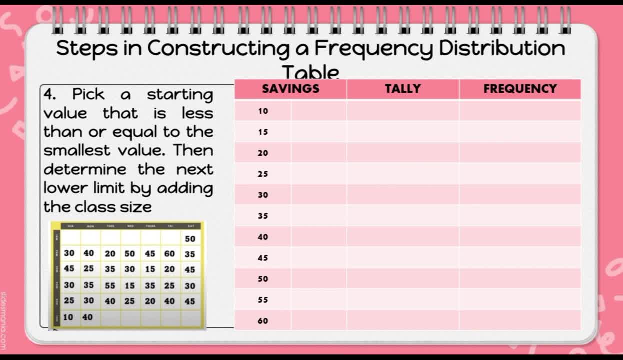 so, as you can see, the lowest value or the smallest value we have is 10, right? so this why we have 10 there in our first row. so again, a row in a table is what we call the interval. so again, determine the next lower limit by adding the class size. so again, since we have already, 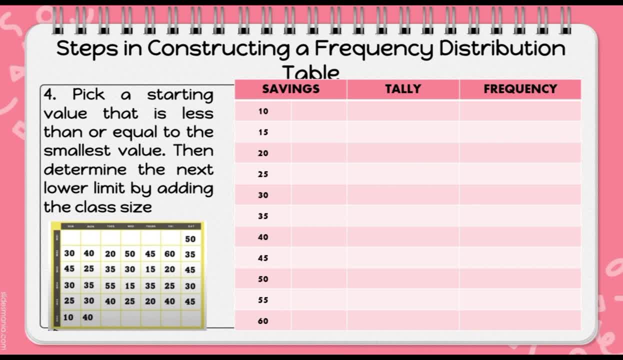 solved for the class size, which is 5, right, we simply add 5 to our first column, first row, which is 10. so 10 plus 5, we have 15. that is why we have 15 in our second row. so 15 plus 5, we have 20. 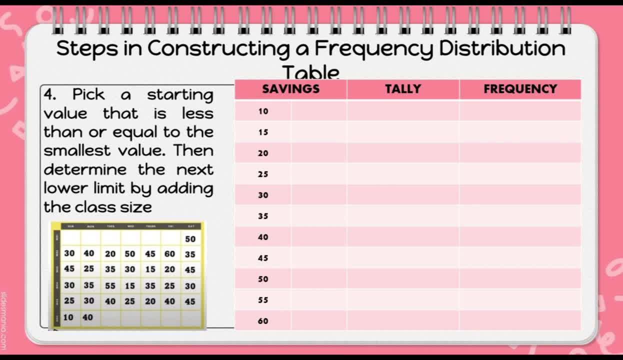 20 plus 5, we have 25, 25 plus 5, we have 30, so so on and so forth. so you have to continue adding 5 until we reach 60, which is our highest value again. so 10, 15, 20 to 60. so this part is what we call the. 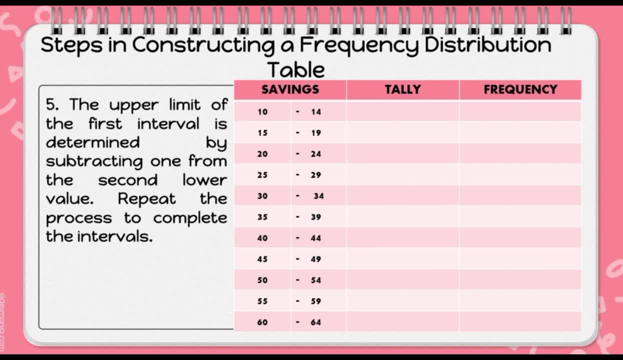 lower limit. all right for our fifth step. we have the upper limit of the first interval. it is determined by subtracting 1 from the second lower value. so repeat the process to complete the intervals. so again in here in our tables. our second lower limit is 15. again, we simply subtract 1. 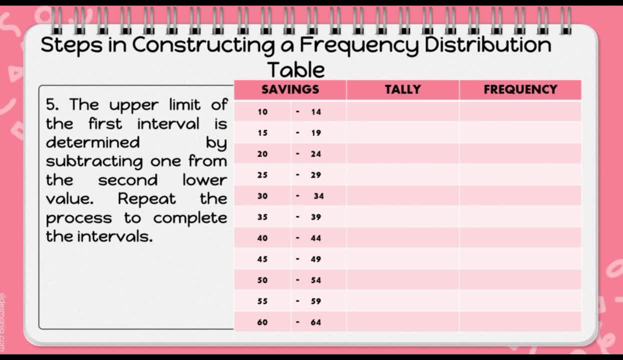 in our second lower limit. so 15 minus 1 is equal to 14.. that is why we have 14 there in our first upper limit. so in order to subtract the first lower limit, we need to add 15 to our second lower limit. So for the second upper limit we have to add our first upper limit by our class size. 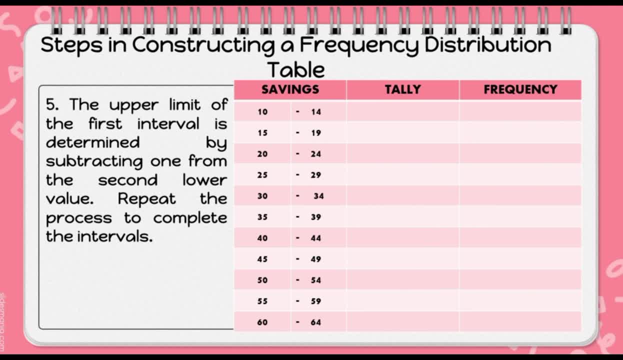 Again, our class size is 5,, right, So we simply add 14 plus 5.. That is why we have 19 in our second upper limit. So 19 plus 5, we have 24.. 24 plus 5, we have 29.. 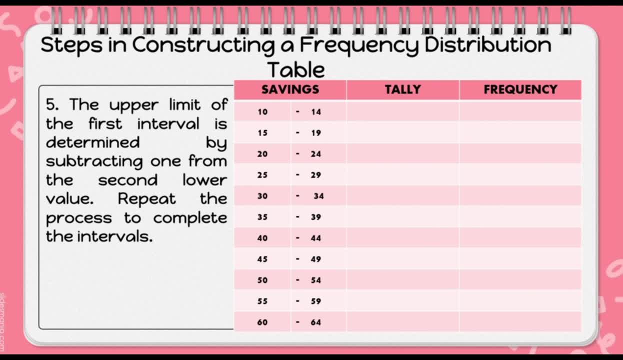 29 plus 5, we have 34. And continue adding 5 until we reach 64. So 14,, 19,, 24,, 29,, 34, until 64. So this part is what we call the upper limit. 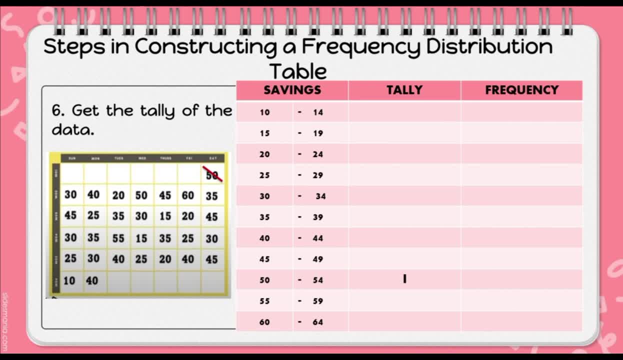 Okay, let's proceed to our next step. We have step 6, get the tally of the data. So here, in this step, we have to be very, very extra careful in tallying the data. So again in our first interval, 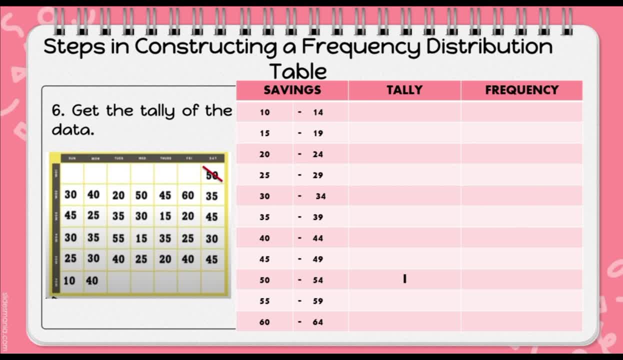 We have 10 to 14. So this includes 10,, 11,, 12,, 13, and 14.. The second interval: we have 15,, 16,, 17,, 18,, 19.. So here in our interval we will tally if our example here belongs to that interval. 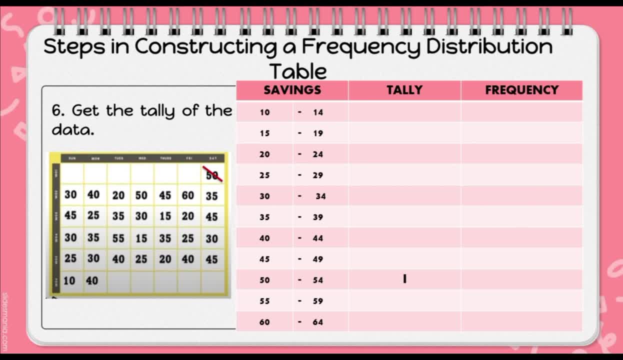 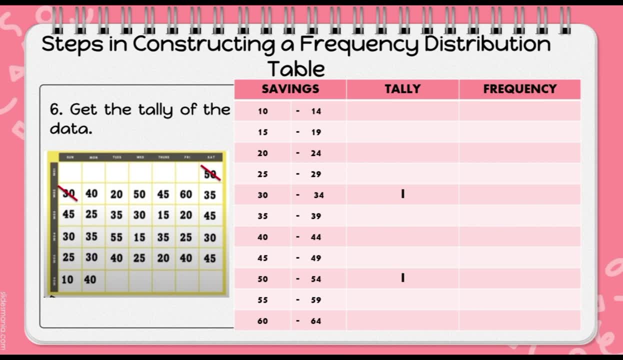 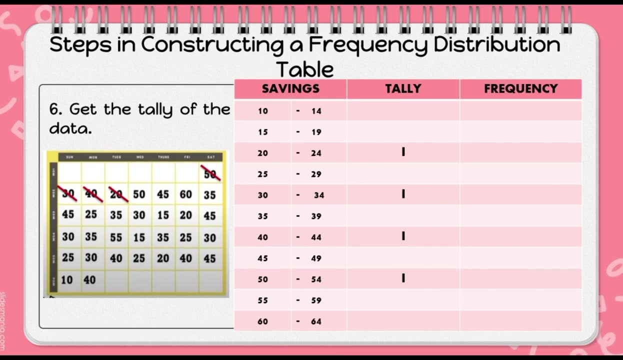 For example, we have 50.. So 50 belongs to 50 to 54.. Next is 30. So 30,, 30 to 34.. So 40,. we have 40 to 44.. 20 belongs to 20 to 24.. 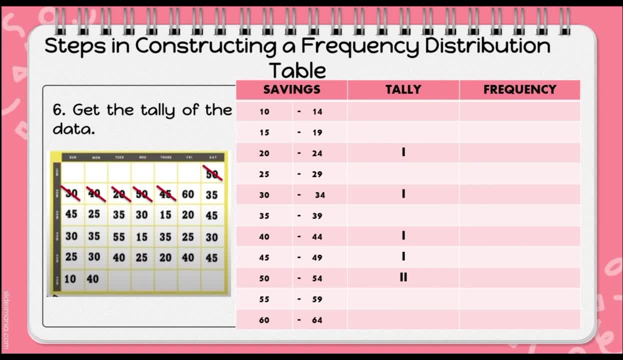 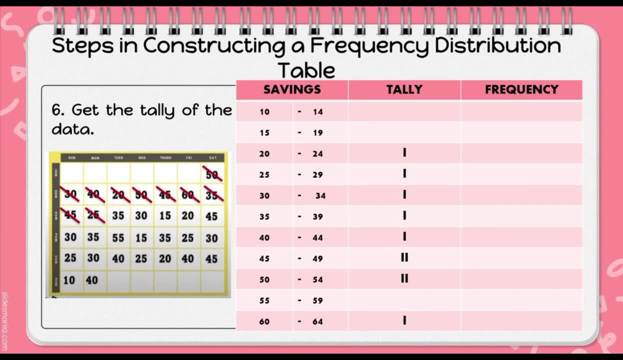 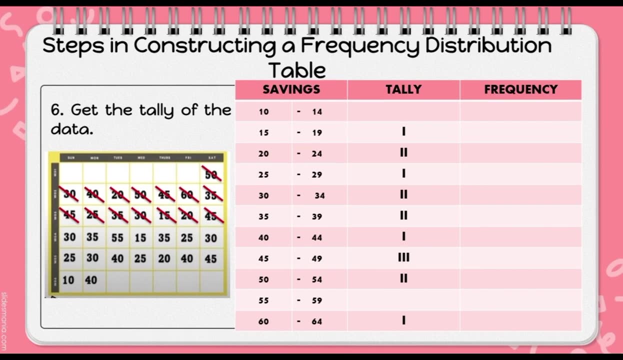 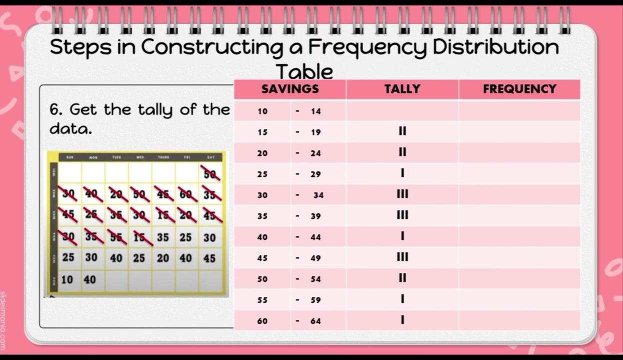 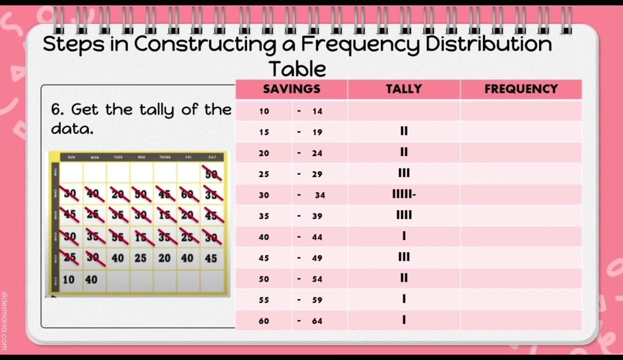 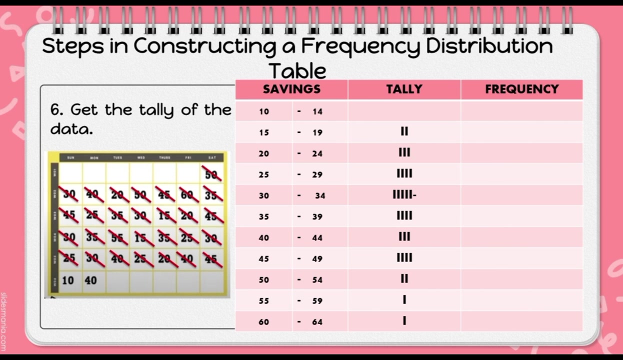 So 50,, 45,, 60,, 35,, 45,, 25,, 35,, 30,, 15,, 20,, 45.. 30,, 35,, 55,, 15,, 35,, 25,, 30,, 25,, 30,, 40,, 25,, 30,, 40,, 25,, 20,, 40,, 40,, 45,, 10, and 40. 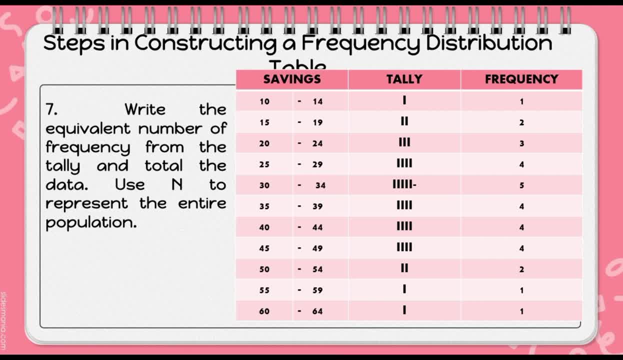 Okay, for our next step we have step 7.. Write the equivalent, The equivalent number of frequency, from the tally and total the data. So use n to represent the entire population. So in solving for the frequency we simply add the tally. 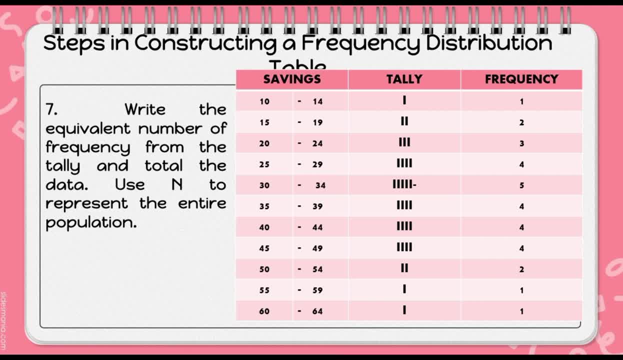 So in our frequency, in the first interval we have 1.. In our second interval we have 2.. In our third interval, we have 3.. In our fourth interval, we have 4.. In our fifth interval, we have 5.. 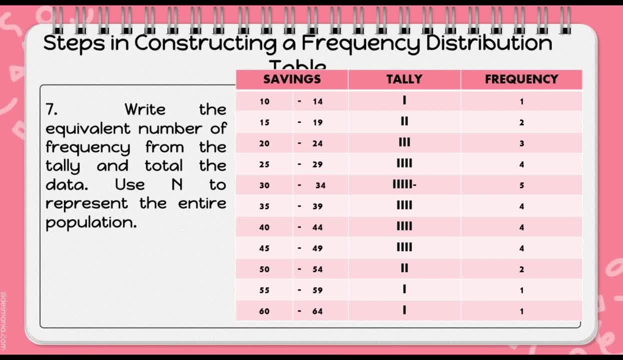 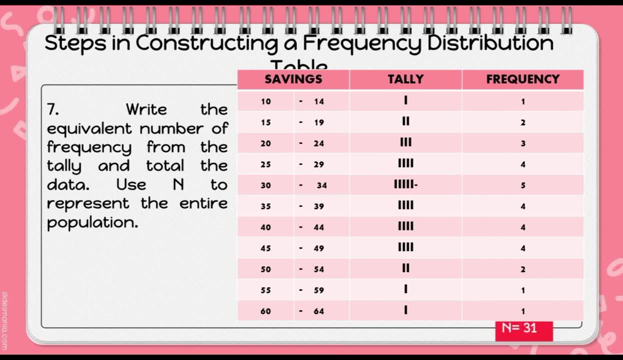 So we have 4, 4, 4,, 2, 1, and 1.. So if we add this all, it will result to 31.. That is why we have n to represent. the entire population is equal to 31.. 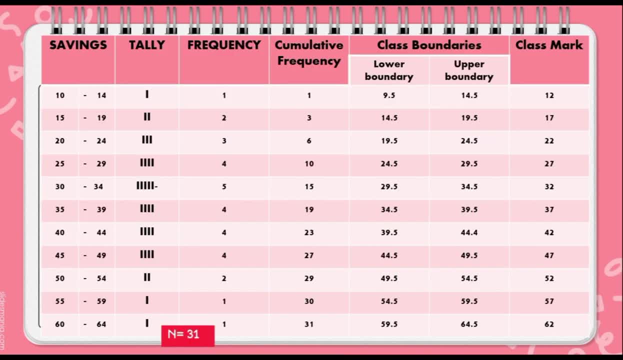 Alright in this table to solve for the cumulative frequency first is you have to look at the first interval in our frequency We have 1.. So this is 1.. This is why in our first cumulative frequency, in our first interval, we have 1 there, right? 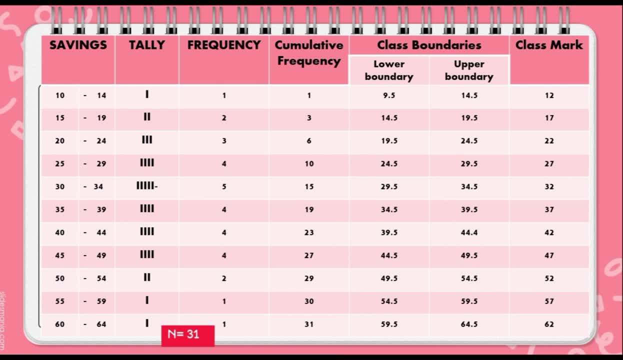 And second step, to get the second interval for the cumulative frequency, which is 3, we simply add the first interval to our second interval in our frequency, which is 2.. So 1 plus 2 is equal to 3.. Again to solve for the second interval. 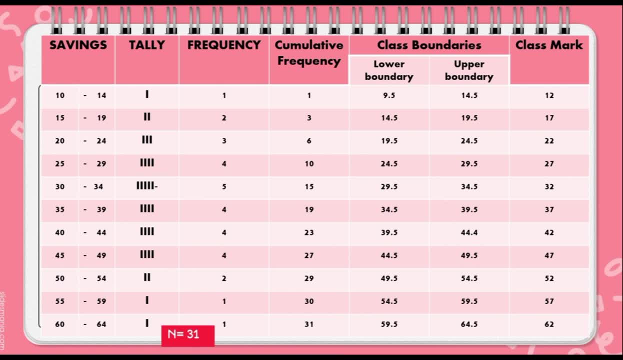 or the second interval for our cumulative frequency. we simply add the first interval, which is 1,, to our second interval in our frequency, which is 2.. So 1 plus 2 is equal to 3.. And repeat the process. 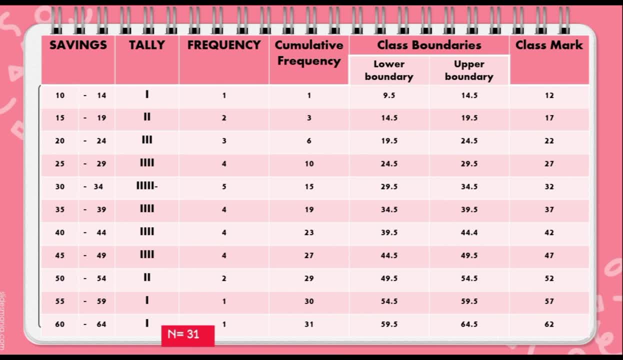 So again 3 plus our third interval in our frequency, which is 3.. That is why we have in our third interval in our cumulative frequency, we have 6.. Again 6 plus 4, we have 10.. 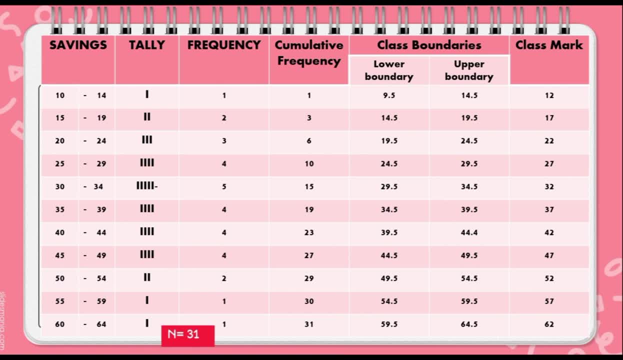 10 plus 5, we have 15.. 15 plus 4, we have 19.. 19 plus 4, we have 23.. 23 plus 4, we have 27.. 27 plus 2, we have 29.. 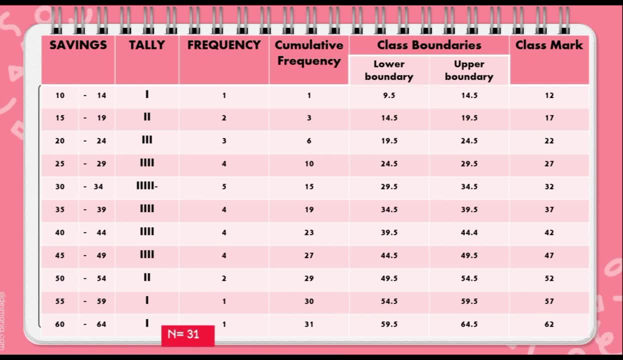 29 plus 1, we have 30. And 30 plus 1, we have 31.. As you can see in the last number in our cumulative frequency, 31 is equal to the total of our frequency, which is n is equal to 31.. 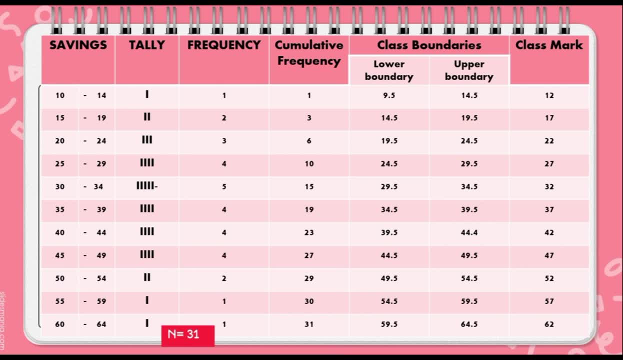 Again to solve for the cumulative frequency. I know some of you are very confused Again, since our frequency here in our first interval, or again in the first row, which is 1, we simply copy 1 in our first row for our cumulative frequency. 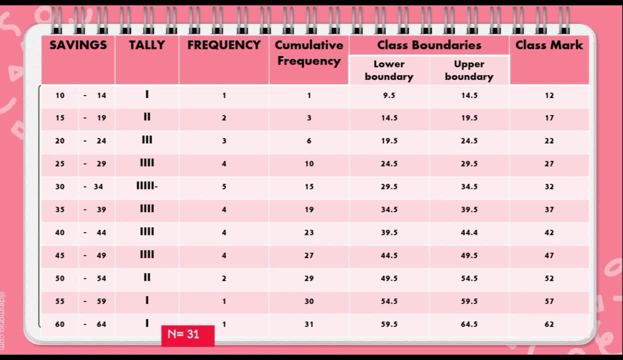 So 1. So 1, since we have 1 here. look at the frequency in our second row, which is 2.. So you have to add that 1.. So 1 plus 2 is equal to 3, right. 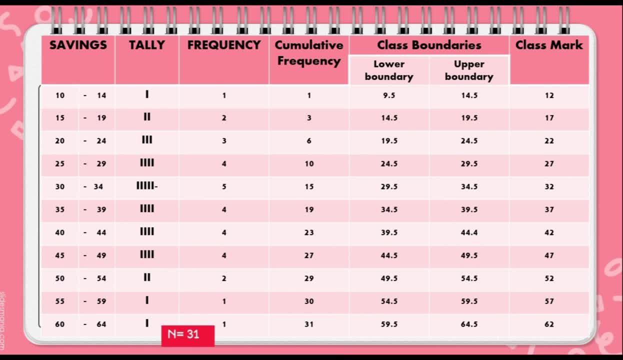 This way we have 3 there in our second row in our cumulative frequency. So again, repeat the process. 3 plus 3 is equal to 6.. 6 plus 4 is equal to 10.. Alright for our class boundaries. 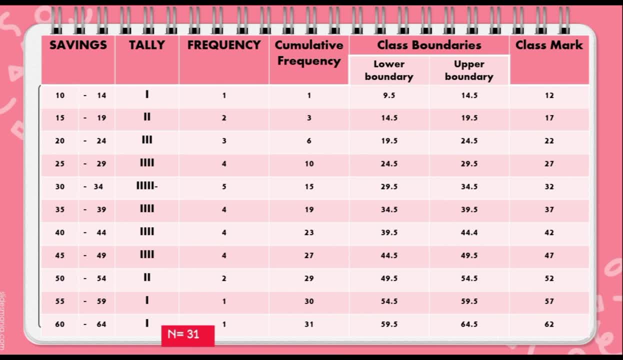 as you can see, it is divided into two parts, Which is the lower boundary and the upper boundary. So, in order to solve for class boundaries, we simply look at the class interval. So, again, in our first class interval, we have 10 to 14.. 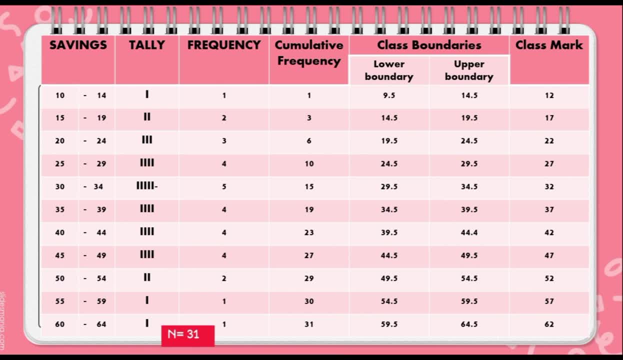 So again, 10 here is our lower limit And 14 is our upper limit. So again, to solve for the lower boundary, we simply subtract 0.5 to our lower limit, which is 10.. So 10 minus 0.5,. 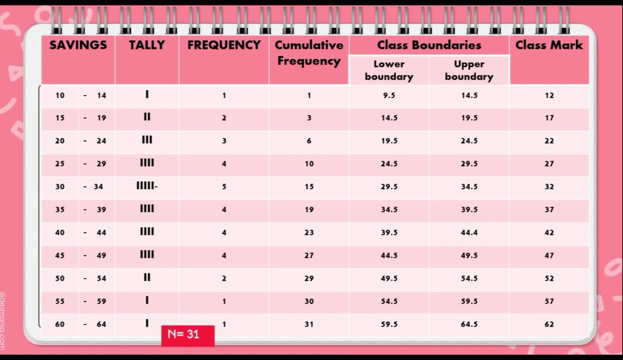 that is why we have in our lower boundary we have 95.. And to solve for our upper boundary, we simply add 0.5 to our upper limit, which is 14 plus 0.5.. That is why we have 14.5 in our upper boundary. 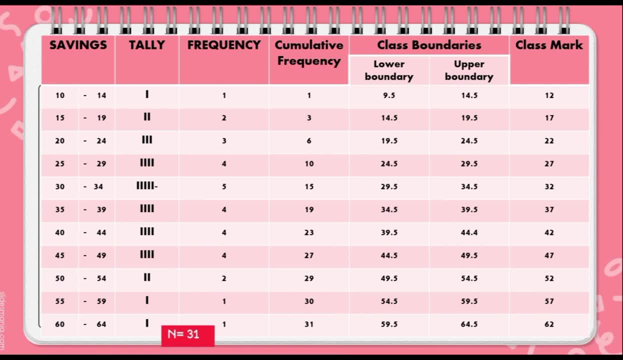 In our second. so 15 minus 0.5, we have 14.5.. And 19 plus 0.5, we have 19.5.. So 20 minus 0.5, we have 19.5.. 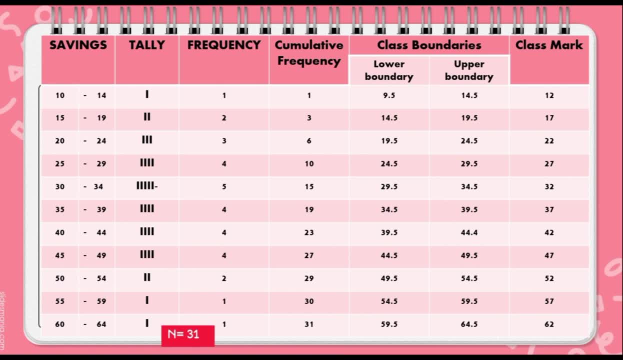 24 plus 0.5, we have 24.5.. 25 minus 0.5, we have 24.5.. And 29 plus 0.5, we have 29.5.. So continue that, adding and subtracting 0.5. 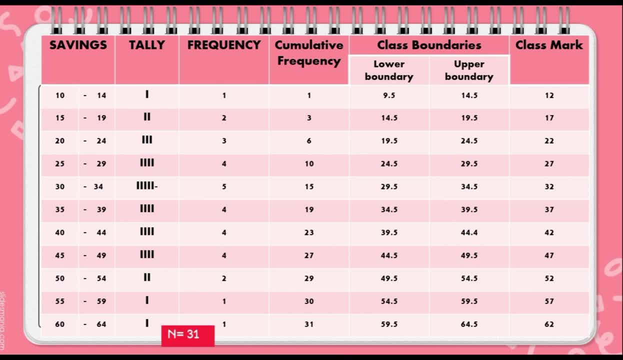 until we reach 50.5 and 64.5.. That is how to solve for the class boundaries. Again, to solve for the lower boundary, we simply subtract the lower limit by 0.5.. And to solve for the upper boundary, 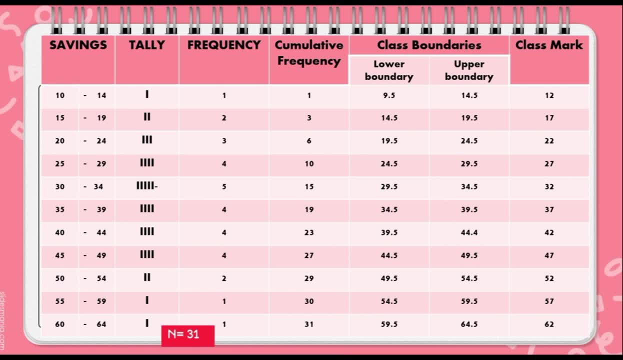 we simply add 0.5 to our upper limit. Alright, in order to solve for the class mark, we simply add the lower limit plus the upper limit divided by 2.. So here, in our first interval, we have our lower limit, 10,. 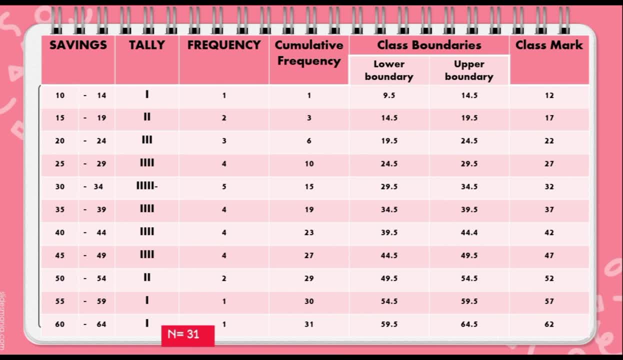 plus our upper limit 14.. So 10 plus 14 is equals to 24.. Divided by 2,, we have 12.. So 15 plus 19 is equals to 34.. Divided by 2,, we have 17.. 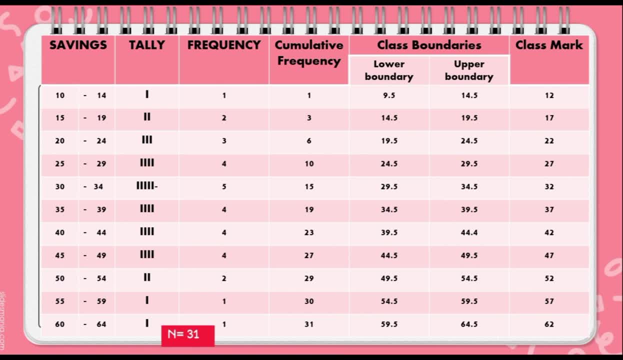 So 20 plus 24, we have 44. Divided by 2, we have 22.. So on and so forth until we reach 62. That is how you solve for the class mark. Again, to solve for the class mark. 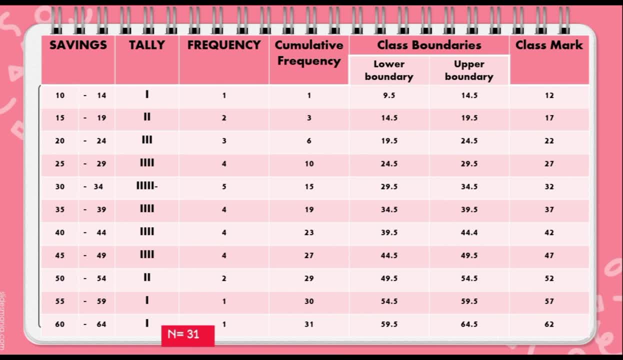 we simply add the lower limit plus the upper limit and divide it by 2..